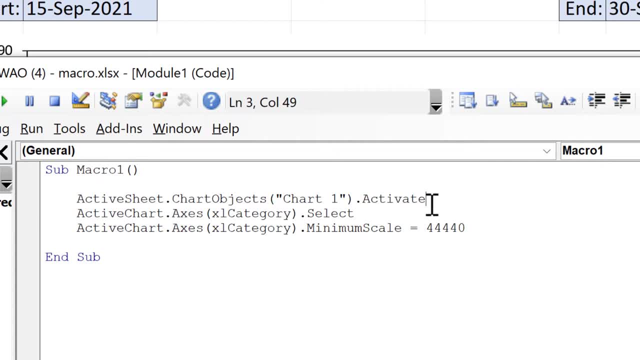 but I don't actually need to activate the chart in order to make changes to it, So I can delete this part here and also the word active, which is part of active chart. on the next line, we do still need to keep the word chart in here, because the chart is actually a thing inside of. 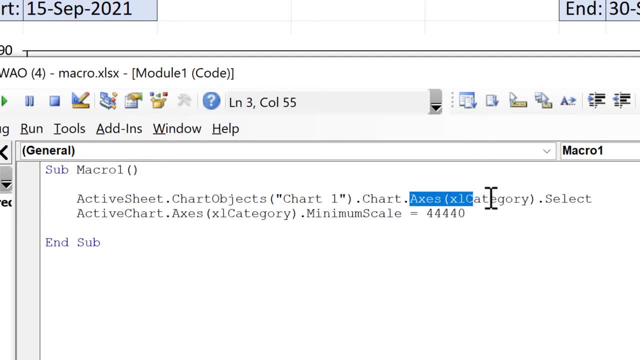 the chart object. then axes- xl category means the x axes and dot select means select the x axes. but again, you don't actually need to select the axes in order to make changes to it. so i can delete this part here. and then also active chart dot axes- xl category on the line below it, as that: 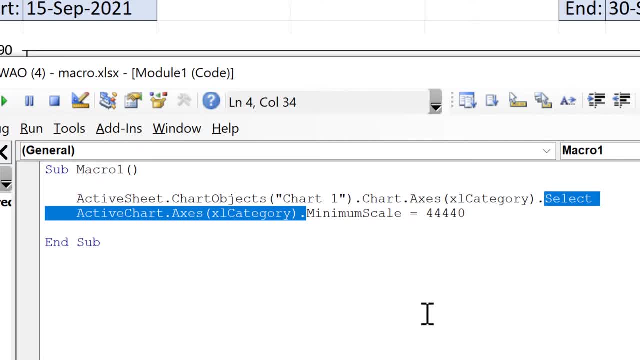 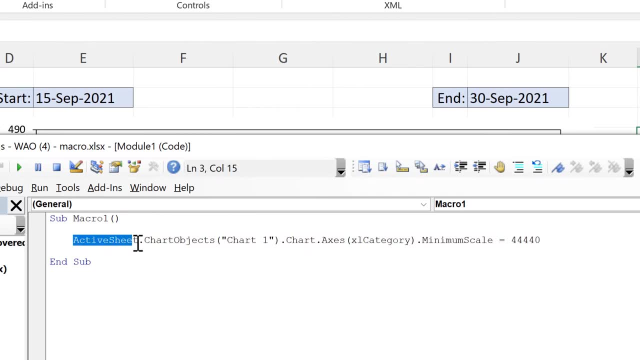 is just a copy of the line before it, and now i have the one line of code that i actually want. so in the active sheet we're looking at the chart called chart one and we are taking the x-axis of this chart and changing the minimum value. 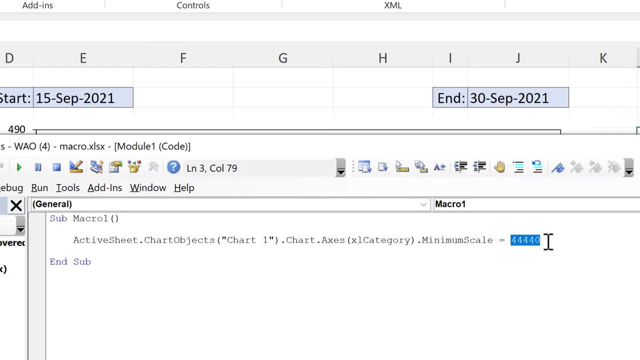 of it to be equal to this value here, but i don't want it to actually be equal to this number. i want it to be equal to the value in this cell here. so in order to do that, i am going to do equals, range, open and close brackets and then in quotation marks i'll put this cell reference. 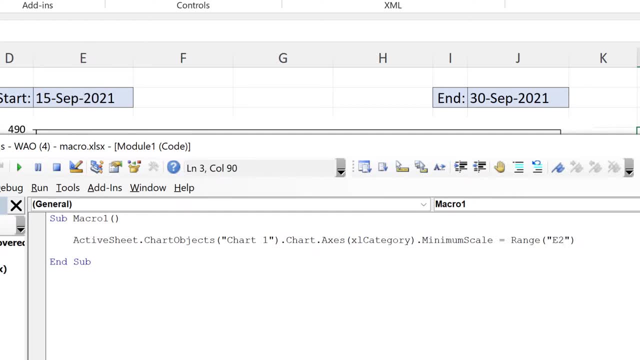 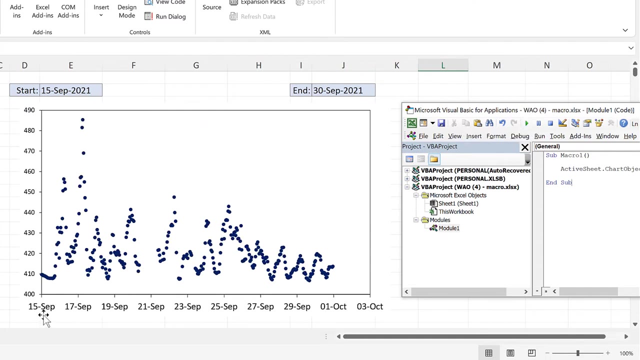 here, so that is e2, and then after this i'll put dot value so it will be equal to the value in this cell. i put in the value in this cell here. now, if i run this macro you'll see that the minimum of the x-axis changes to the 15th of september. 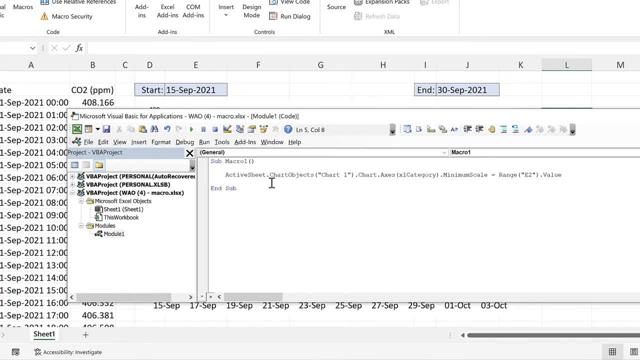 but instead of running the macro each time, i want for this line of code to run automatically whenever the value in this cell changes. and in order to do that, i'm going to copy this line of code here and double click on sheet one, which is the sheet. 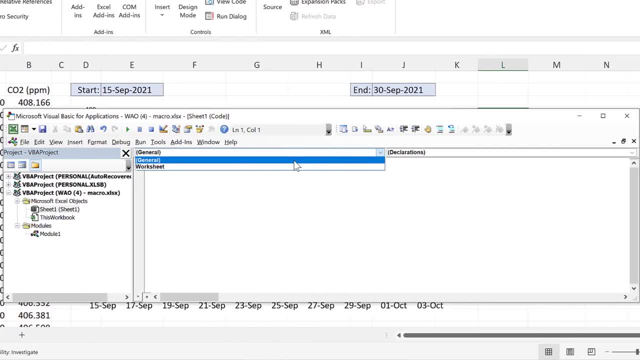 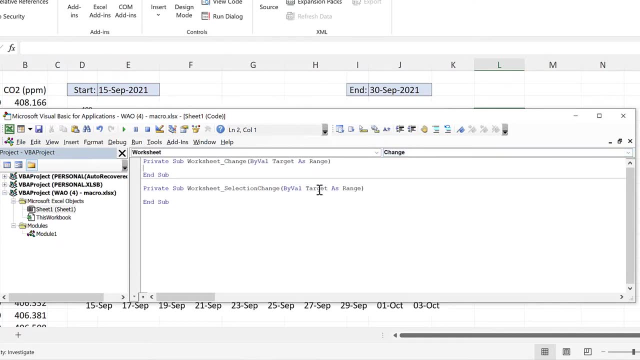 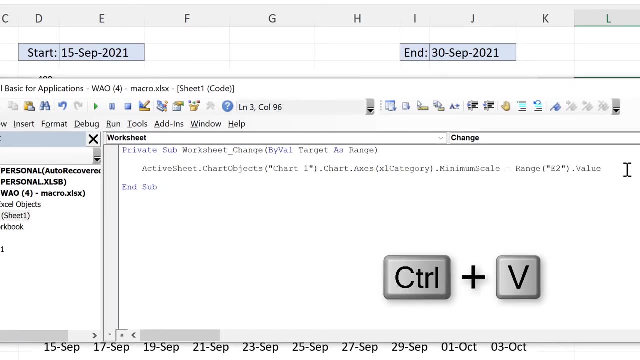 that I am currently in and then change this here to worksheet and use this drop-down list here to select change, then we can delete this part and paste in here the line of code that I just copied now. at the moment, this line of code will run every single time anything is changed in the worksheet, but I want. 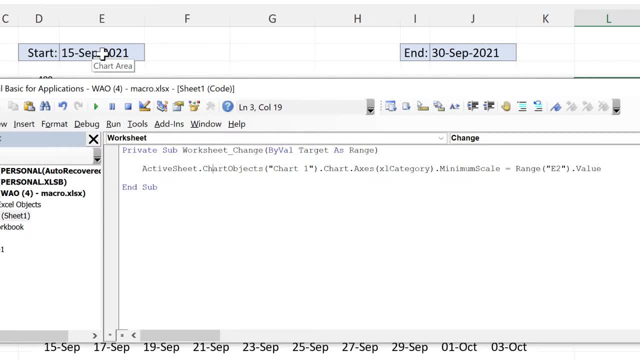 it to run only when the value in this cell is changed. so in order to do that, I need to add in an if statement and I already have the value up here called target. so I'm going to do if target dot address and address is just another way. 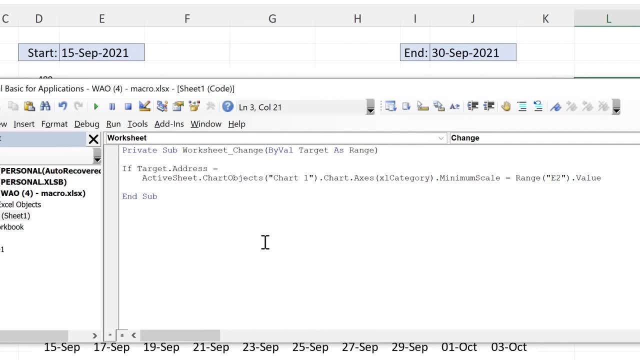 of saying the cell reference is equal to e2 and e2 needs to have dollar signs around it and it also needs to be in quotation marks. so I'm saying if the value in e2 changes, then I want to run this piece of code and then I need an end if after this. now, in order, 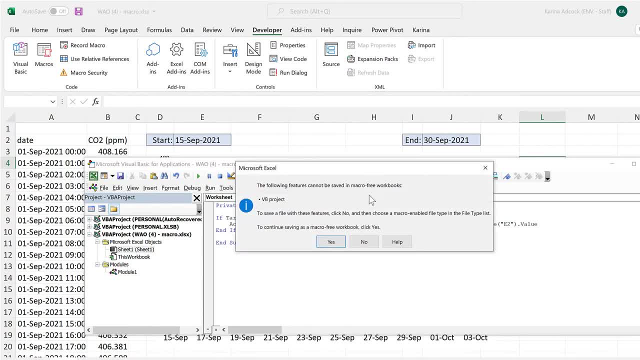 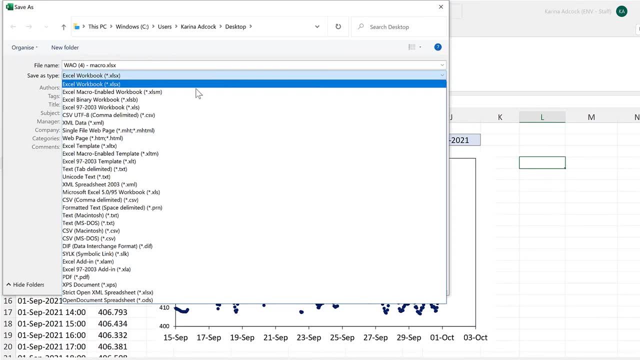 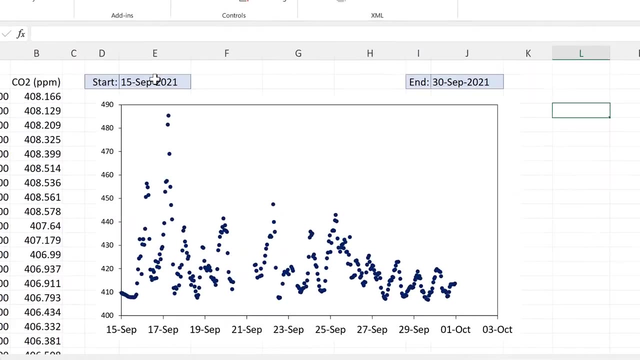 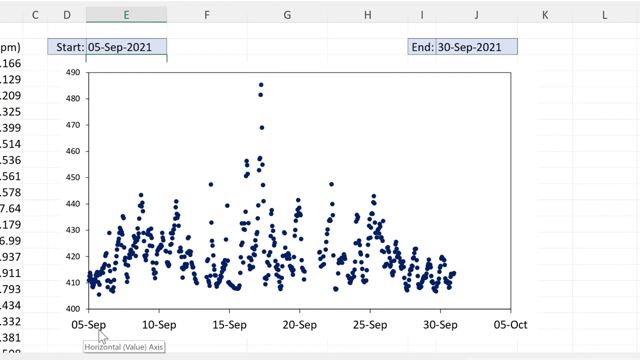 to save this, it has to be saved in a macro enabled workbook. so I'll select no and then change the save as type to a macro enabled workbook and save, and I can change the value in this cell here and the minimum of the x-axis will change. now I also want to do the same. 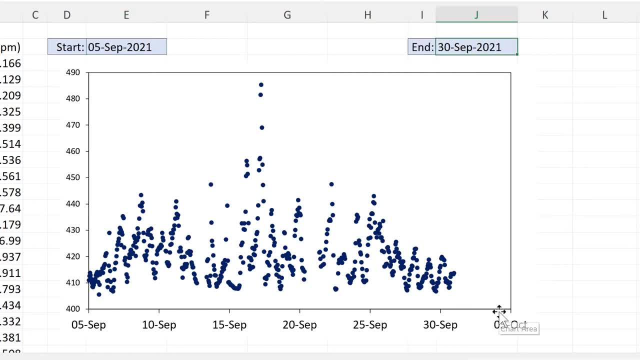 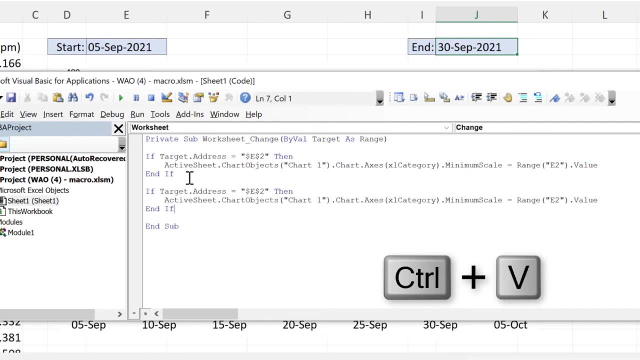 thing for this value here, but this time changing the maximum. so I'm going to do a copy of this if statement here and paste it down here, and then this time we'll change e2 to j2 instead, and instead of changing the minimum we'll be changing. 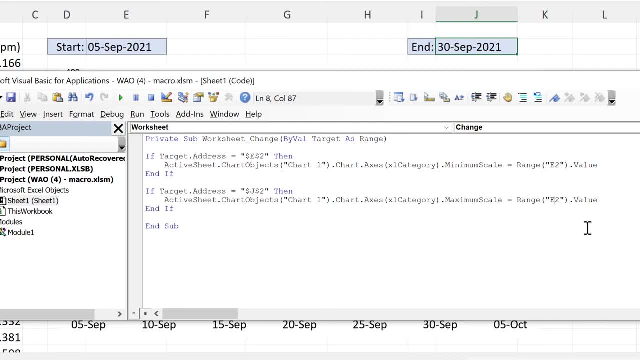 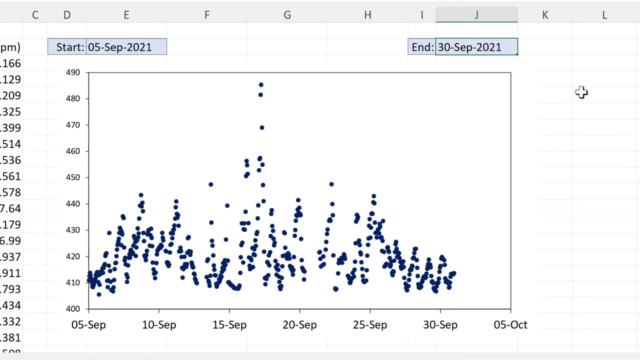 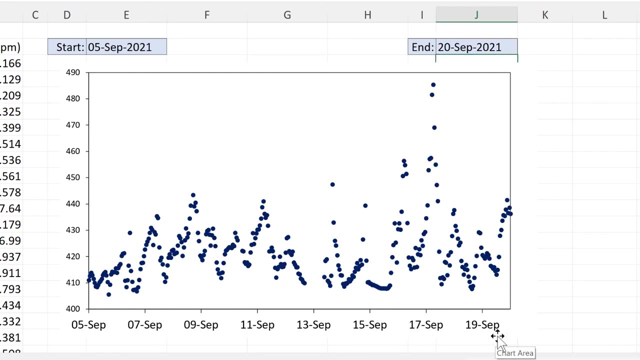 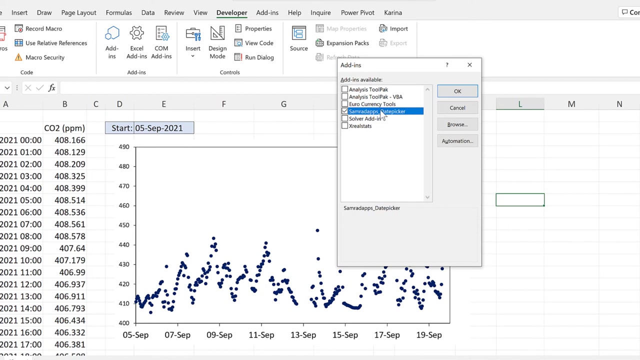 the maximum. and then again here we need to change this to j2 and then we can save this. and now if I change the value in this cell, the maximum of the x-axis will change. now I'm also going to go to Excel add-ins and tick the date picker add-in and okay. and now if I click in any cell,